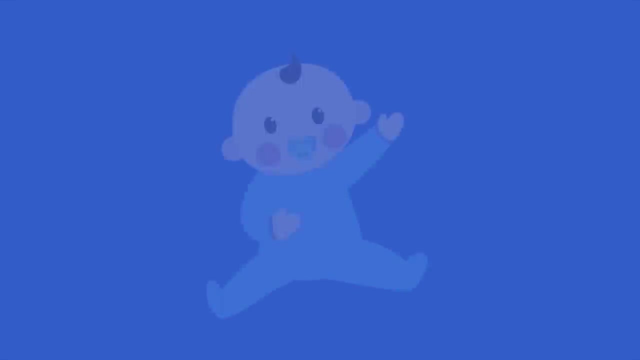 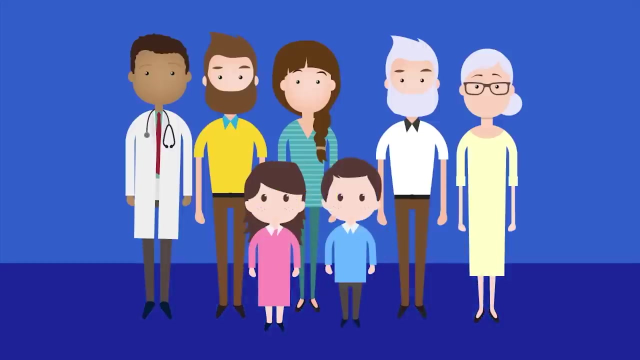 From the moment we're born, we begin to develop our identities. Who are we, What should we care about And how should we relate to all these people around us? As it turns out, the way each of us answers these questions largely depends on the culture we grow up in. One major difference: 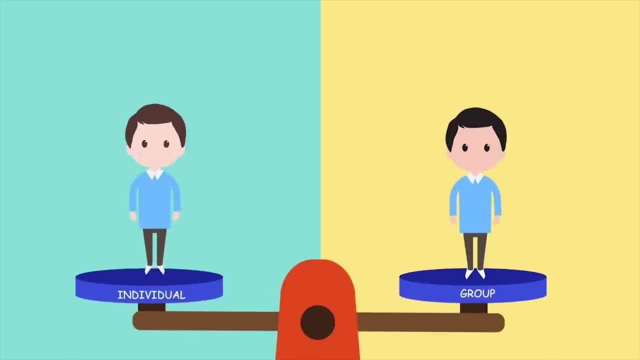 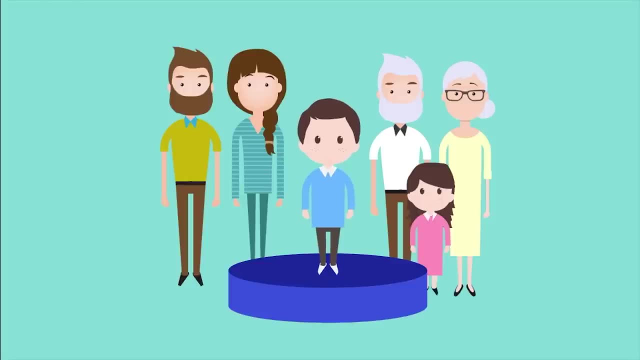 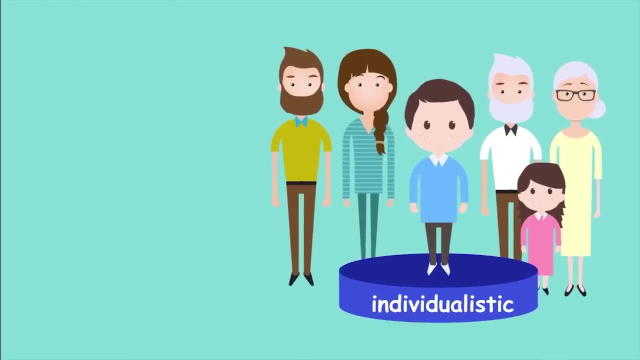 between cultures in the East and the West is how they view the individual in relation to the group. Some cultures tend to place more importance on the individual. They're known as individualistic or me societies. Many Western societies, including those in the United States, Australia and large 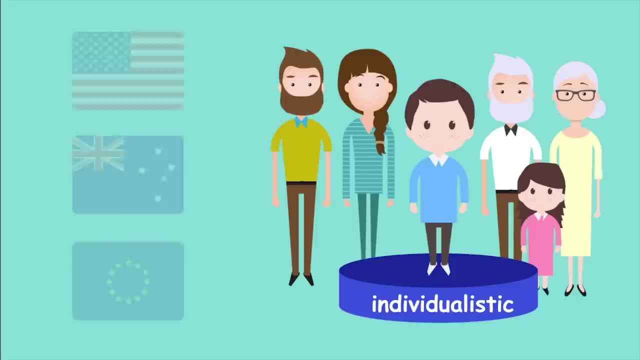 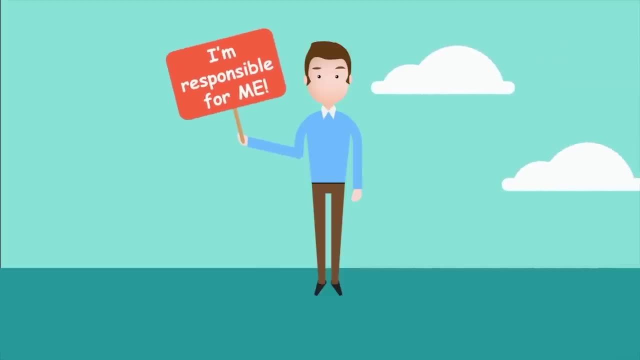 swaths of Europe are considered me cultures. People in a me culture believe each individual is responsible for their own well-being. Their circle of responsibility extends only to their immediate family members. Some cultures tend to place more importance on the individual. They're. 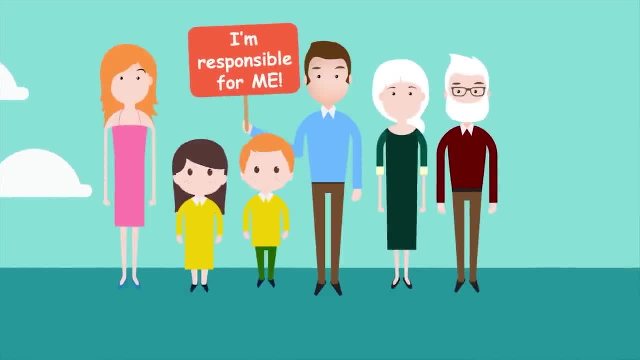 known as member settings and lingere aideribels or spots to be prepared. Juvenile and breeding 지� SASEI N인지ai are both familiar and well in terms of culture. We refer to them as members, parents, spouses, children. They view the responsibility to others in society as limited. 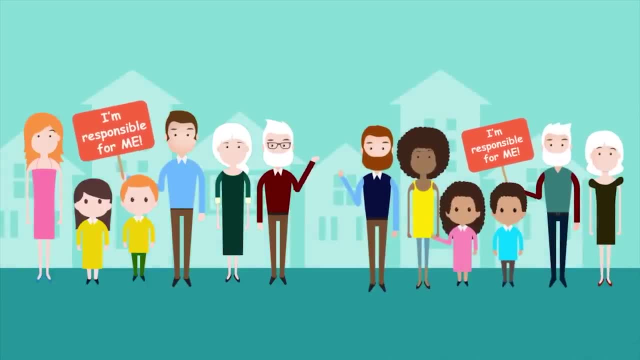 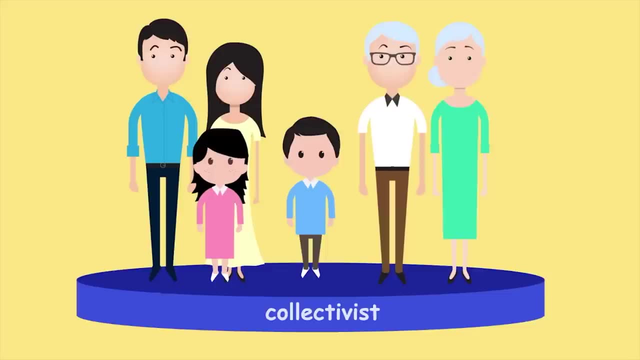 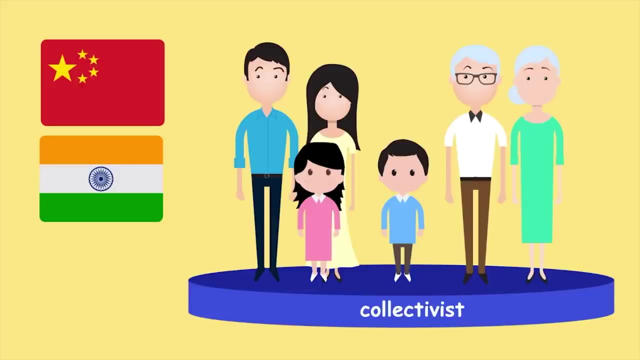 After all, they're also individuals who should be taking care of themselves. On the other hand, some cultures place more importance on the group. They're called collectivist societies or WE cultures. Many Eastern cultures, including those in China, India and Japan, are considered 있 정서생활és. These are so called as part of a collective. 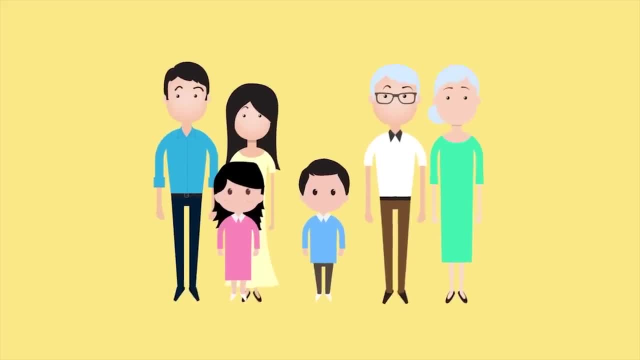 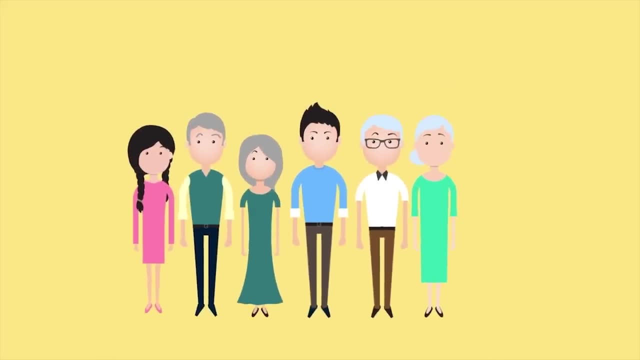 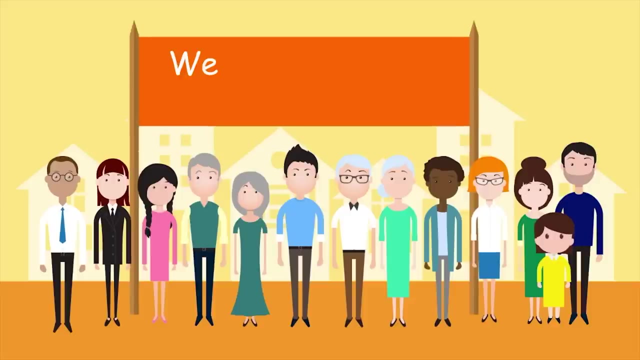 considered we cultures. People in a we culture prioritize strong social ties and belonging to a larger group. These groups might include classmates, neighbors and extended families. They strive for group harmony and believe the individual should make the best decisions for the overall well-being of their group. If you 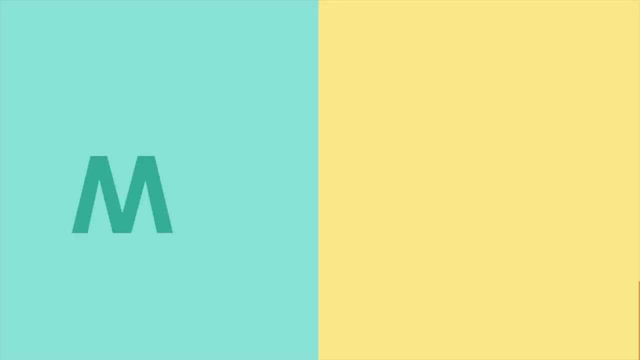 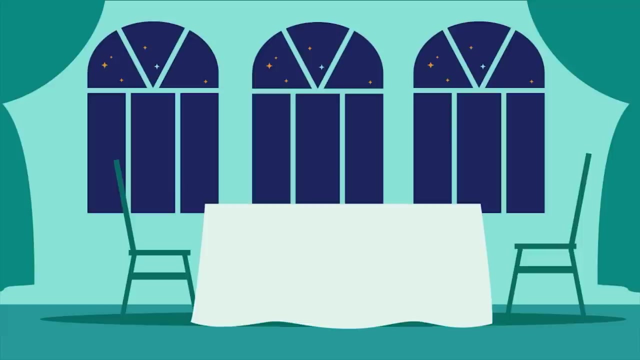 take care of the group, they'll take care of you. So how does this me versus we difference shape our behavior? As it turns out, this seemingly subtle distinction has some surprising effects. Imagine two families each go out to dinner. The family from a me culture might consist of just four people: two. 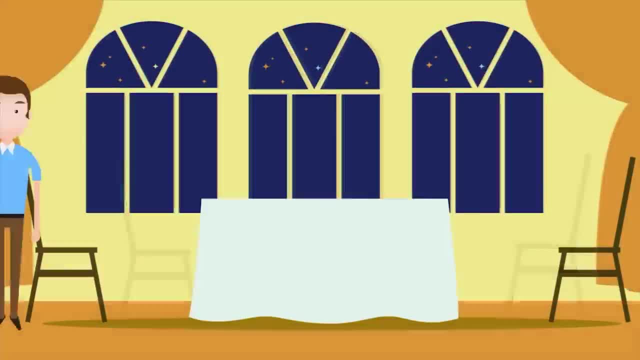 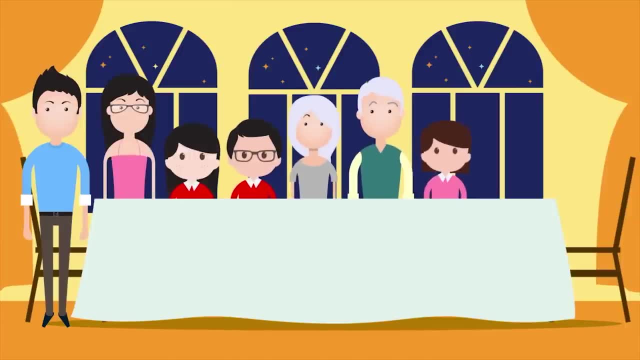 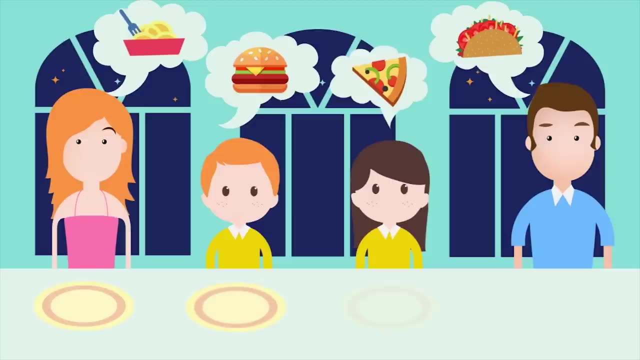 parents and their two children. The family from a we culture would need a much larger table to make room for two children, their cousins and multiple sets of parents and grandparents. At the me table, everyone would order the specific meal they wanted When the 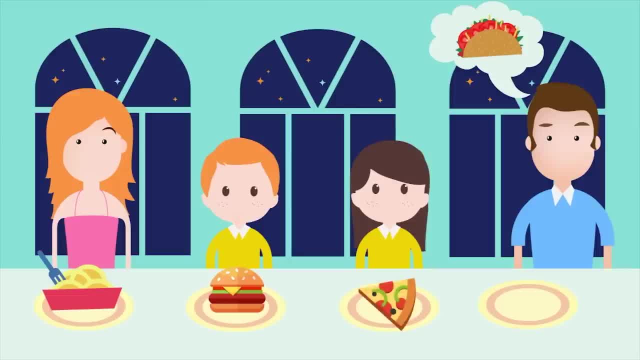 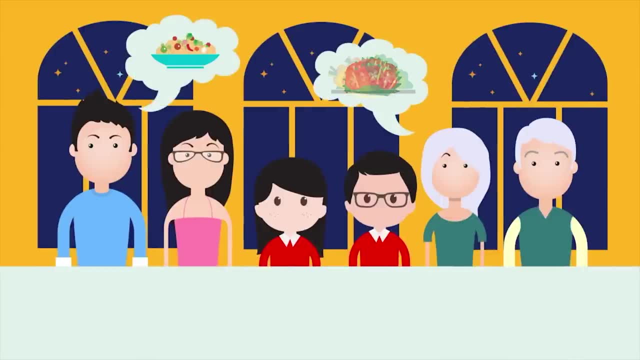 food comes. they may trade a bite or two, but for the most part each person would eat their own meal At the we table. on the other hand, multiple dishes would be ordered for the whole table. They would be placed in the center and all members 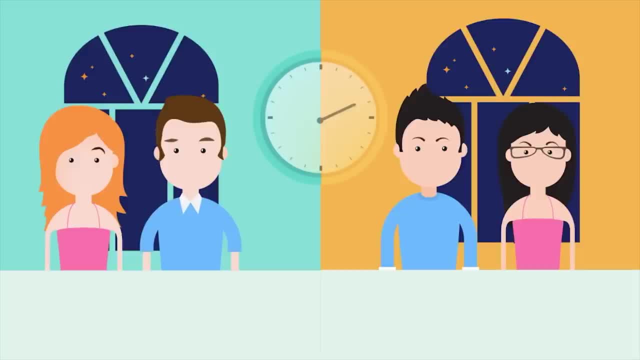 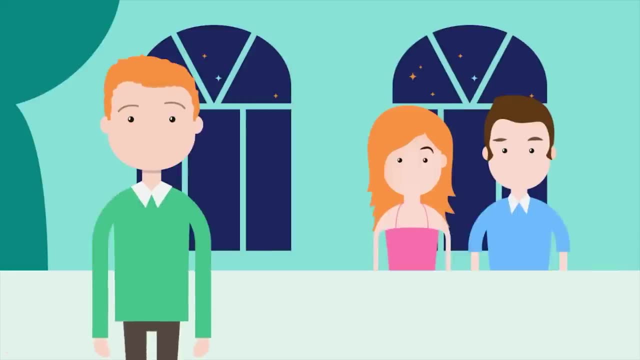 of the family would share them. Now, let's say a family member was running late. How is each table likely to respond? At the me table, people are expected to be masters of their own fate. So when teenage brother Lee arrives late, the 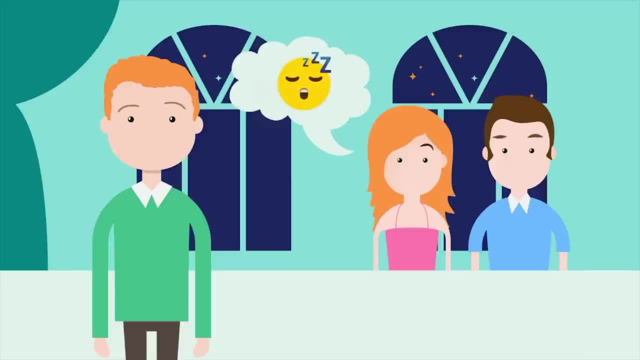 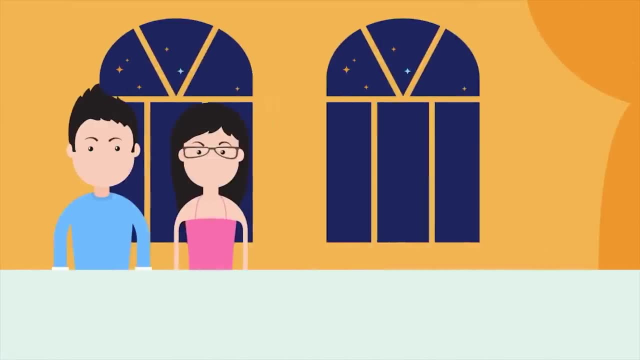 family is more likely to attribute his tardiness to some fundamental aspect of Lee's personality, like assuming he is lazy or irresponsible At the we table. on the other hand, they're more likely to see Lee's behavior as part of a larger context. Rather than blaming him for being lazy, they may assume external. 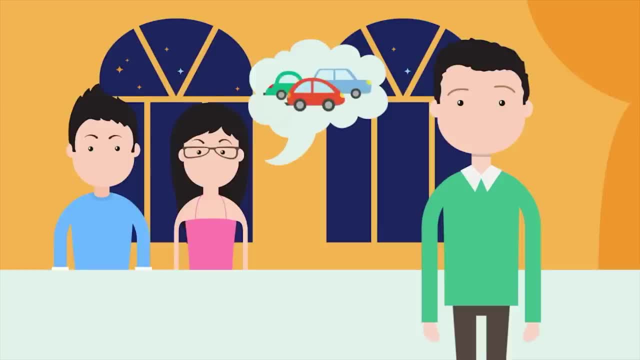 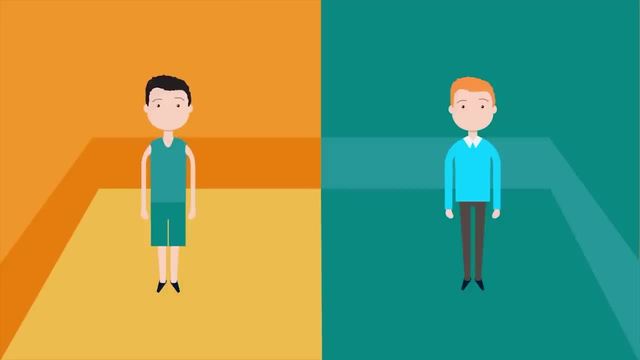 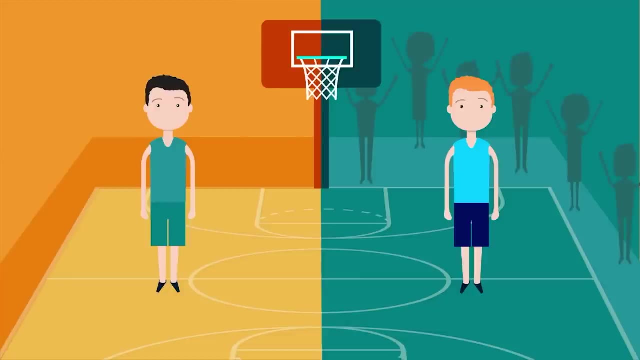 factors were involved. Maybe there was an accident on the road and Lee got caught in bad traffic. This tendency to either credit the individual or the larger context applies to positive things too. Say, Lee was coming from a basketball game where he scored a game-winning shot At the me table. Lee would be celebrated as the 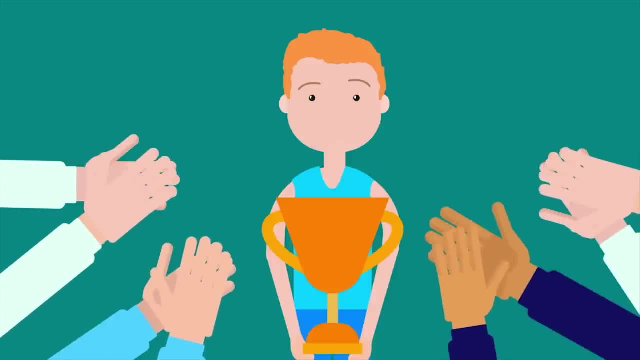 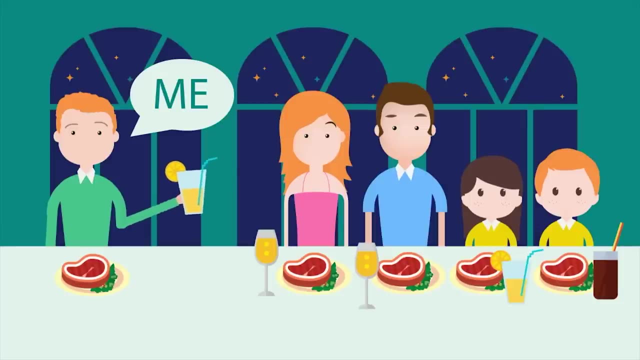 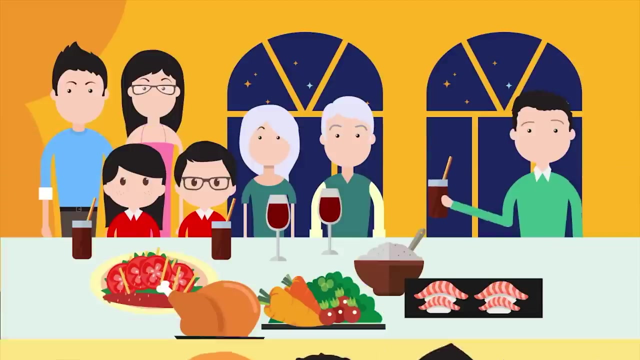 hero. His individual action won the game for the whole team. In a celebratory toast, Lee would likely speak about how his hard work, determination and focus led him to this moment. Meanwhile, at the we table, the team's overall victory would be celebrated. Lee's toast would more likely. 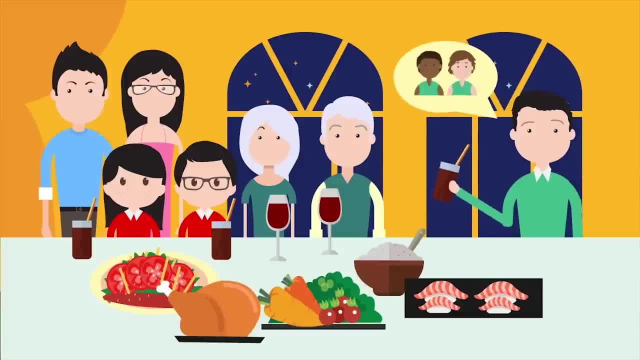 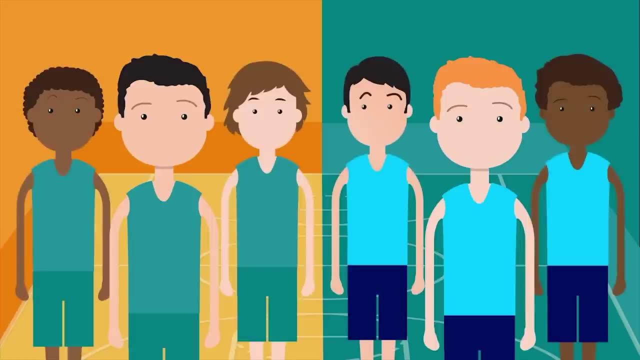 focus on how his teammates, coaches and mentors led to the team's success. He may even mention a larger context, like the support of the team's school administration or fan base. Both of these viewpoints are true. Lee's action secured the victory, but the team's effort won the game. There is no